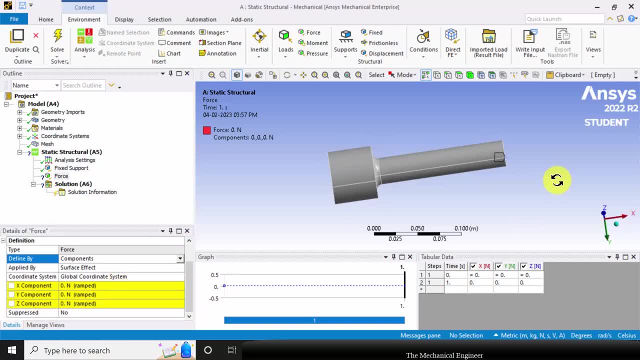 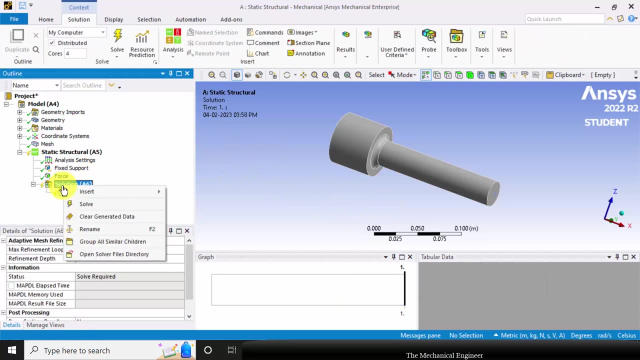 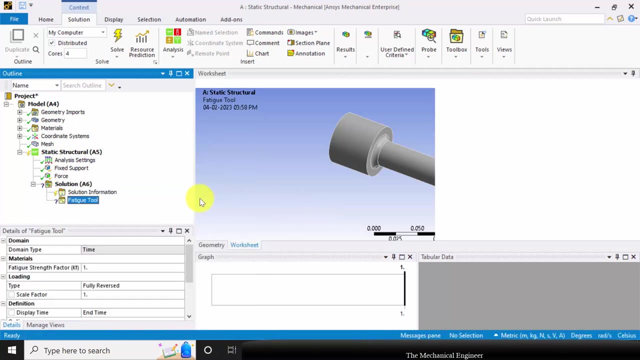 component. So I am choosing component and I am applying a load in the y direction. Now the magnitude of the load is 1000 Newton. Now right click on the solution, choose insert, go to fatigue and insert the fatigue tool. So once you click the fatigue tool you will. 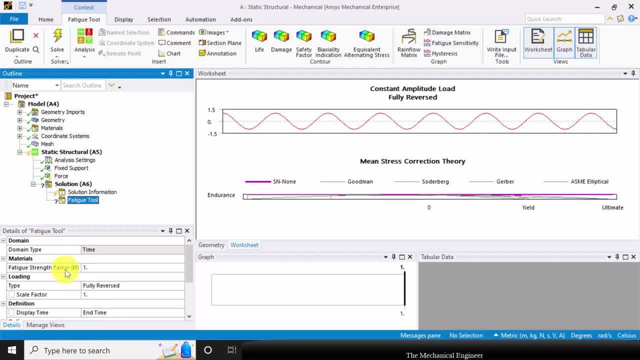 have many options here. So one is fatigue strength factor, Kf. So in our case there is no Kf. So, as I have mentioned, I am proceeding with the 1. Then in the type type of loading we have, fully reversed, and then zero based. Zero based means it will start from 0, not exactly. 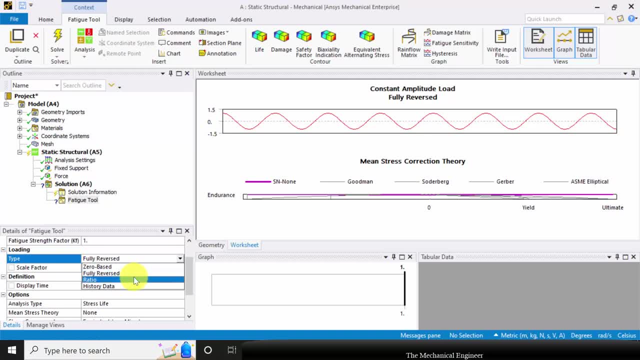 0,, somehow around 0. Then ratio means we can provide some ratio between the maximum and minimum value. Histored data means we can provide the trend of the curve. So I am continuing with the fully reversed And I am going to find out the. 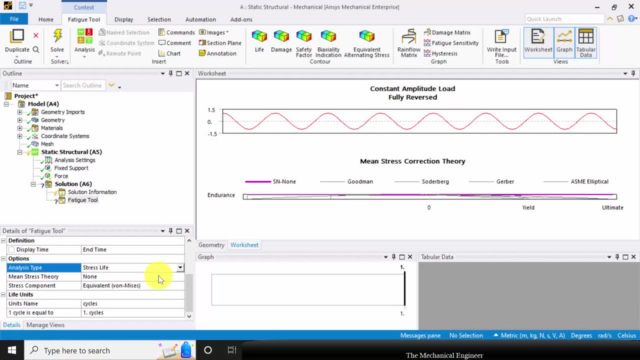 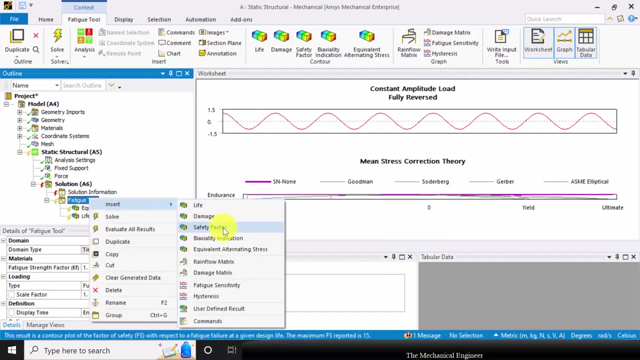 stress life. so you can choose stress life or the strain life. now in the stress component there are standard theories are available, so i'm choosing equivalent one: miss stress. now right click on the fatigue tool and select insert. and i want equivalent alternating stress also, i need life. i'm also inserting the safety factor. now right click on the solution and click. 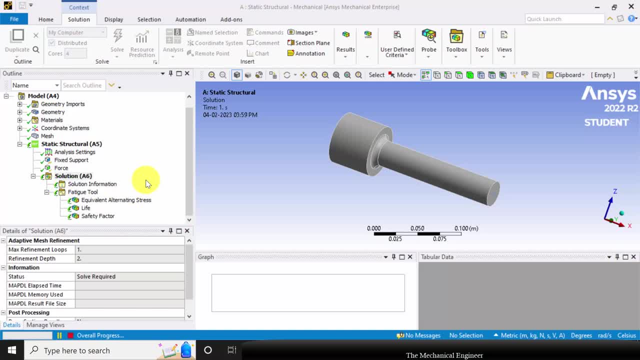 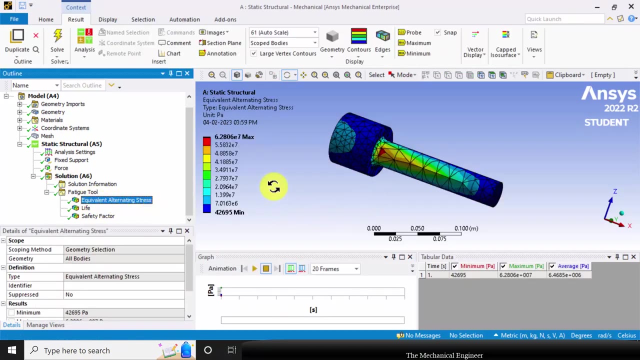 solve now. you can click the equivalent alternating stress and the maximum stress will be equal to the equivalent alternating stress and the maximum stress will be equal to the equivalent alternating stress is of 6.28 e power 7 pascal and you can animate like this: